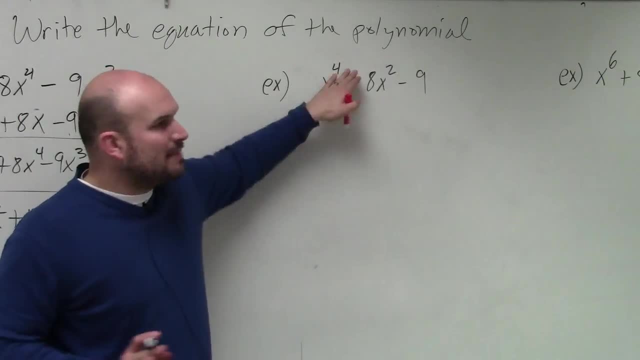 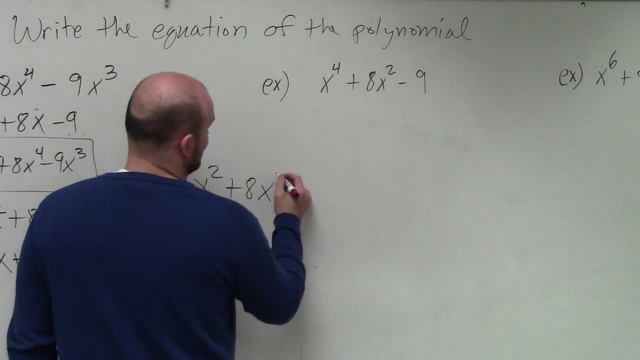 have something like this where you can't factor it out. let's forget about the powers for a second and let's just factor out what we know how to factor. We know how to factor a trinomial when it's a quadratic. Everybody agree with me: We understand factoring quadratics. 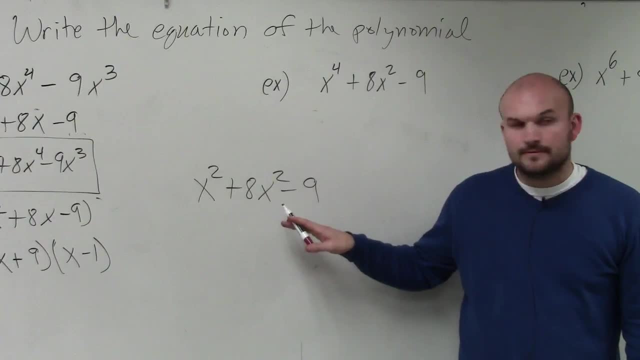 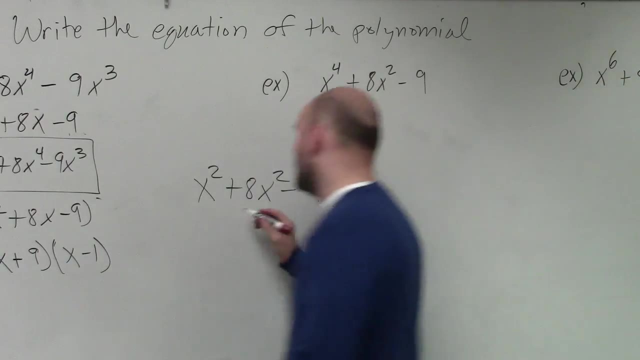 when it is in this format. Okay, So now I'm just writing this down. This is the same numbers, but with x squared. You agree with me? Yes? Now, when we go ahead and factor this, I have x plus 9 times x minus 1.. 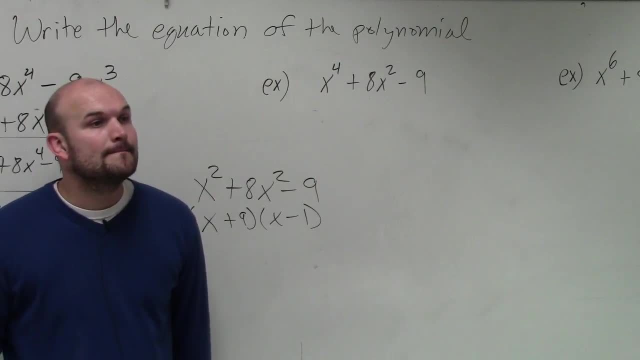 Wait, what's bugged? We didn't write it that way. Huh, I'm trying to explain, but I have some other people that are not paying attention, so it kind of gets a little difficult. Yes, I'm not trying to get Ian to bug, though. 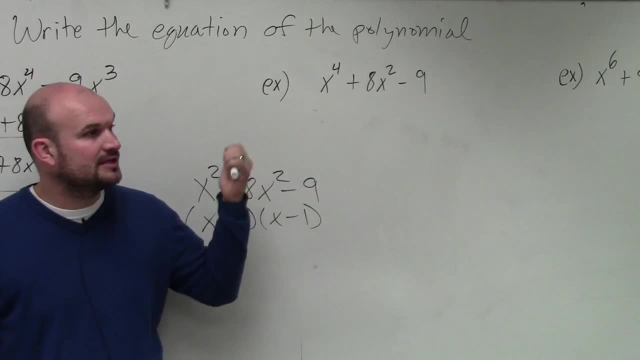 I'm going to explain how to do this problem, but if that's something that's an emergency, then you can take care of it. So we have x squared plus 8x minus 9.. All right, Do you guys agree with me, though, that these two problems 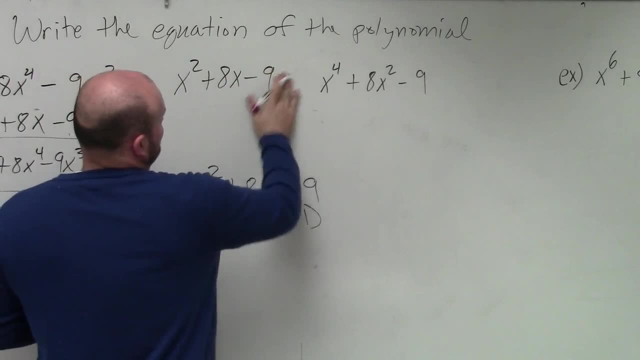 Here. let's do it this way: x squared plus 8x minus 9.. So when we factor this, I get x plus 9 times x minus 1.. Do you guys agree that these problems are very similar to each other? 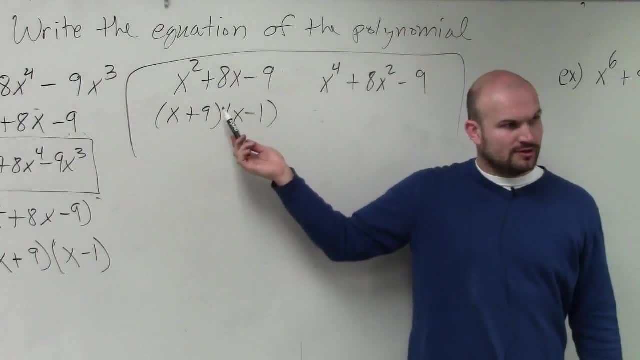 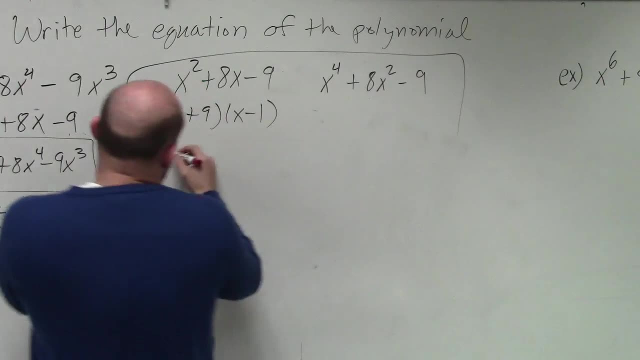 They're very similar to each other. This one is like the algebra 1 quadratic. This one is raised to a power 4, right Now. but what I want you guys to understand is: when we apply FOIL, you multiply the first two terms, you get x squared. When you multiply the last. 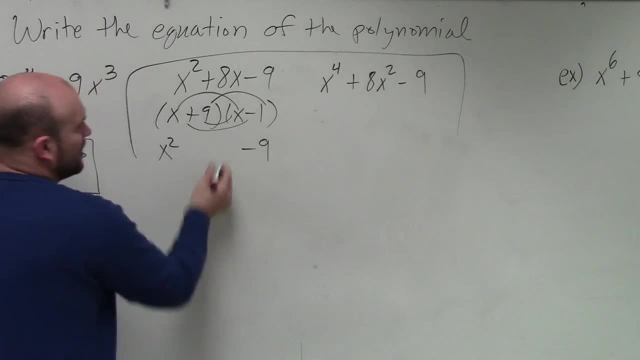 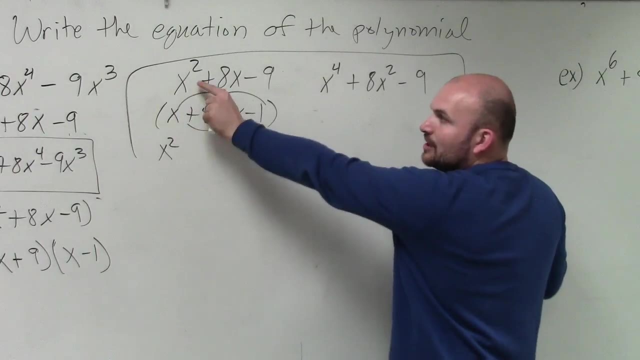 two terms, you get negative 9, right, The middle terms are what combine to give us 8x. So what I want you guys to understand is the factors. the first two terms of the factor give us x squared. The last two terms of our factors give us negative 9.. So in this, 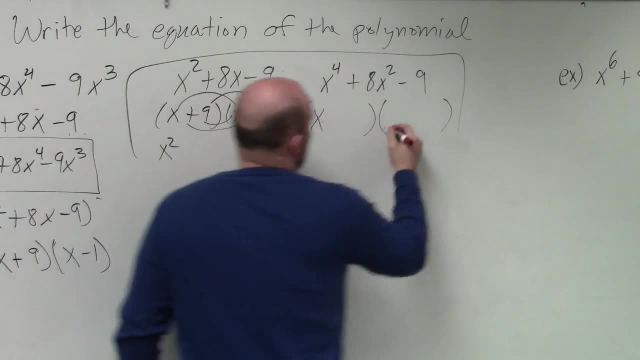 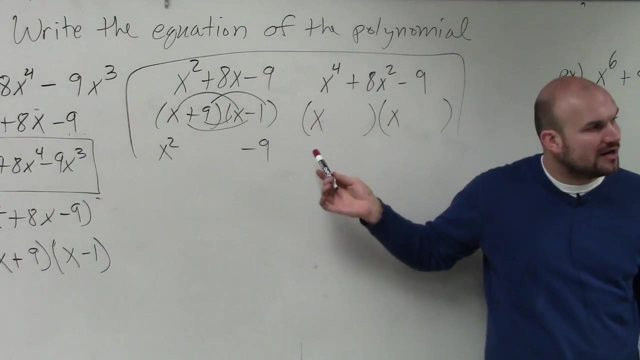 example, I can't use x and x, because x times x gives us x squared. x times x does not give us x to the fourth. However, if I change the power of x, I can get x to the fourth. So